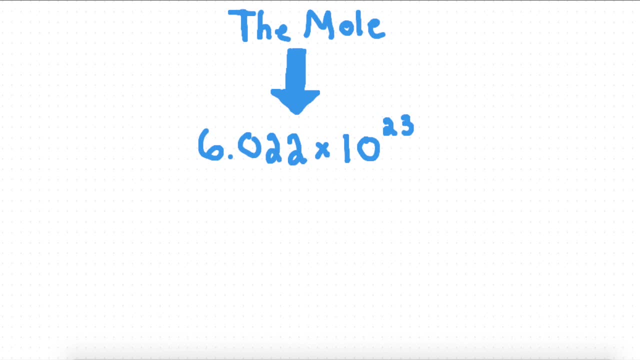 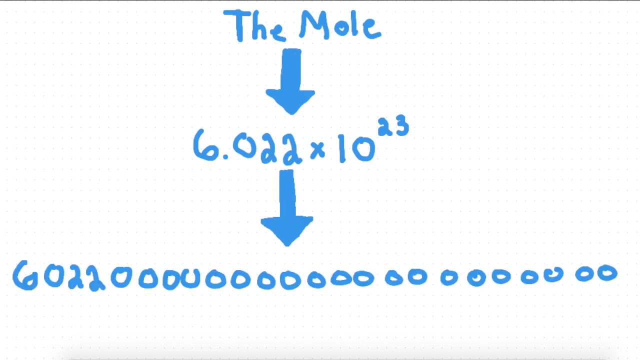 times 10 to the 23rd. That's a really big number and to show you how big it is, we'll show it to you right over here, right now. Yup, there it is: 6.022 with 20 zeros after. 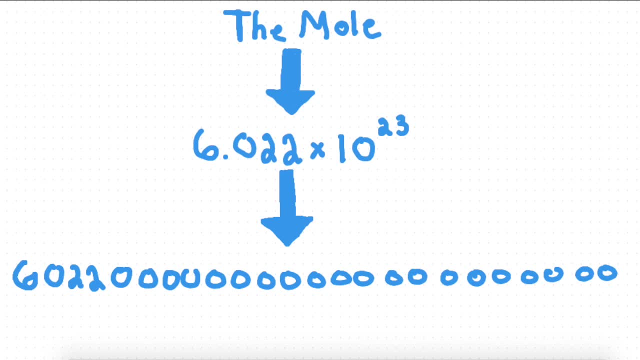 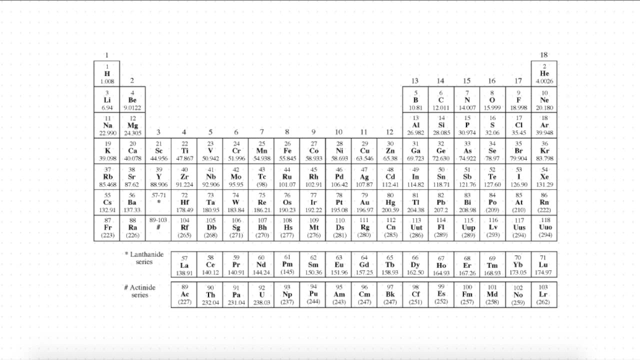 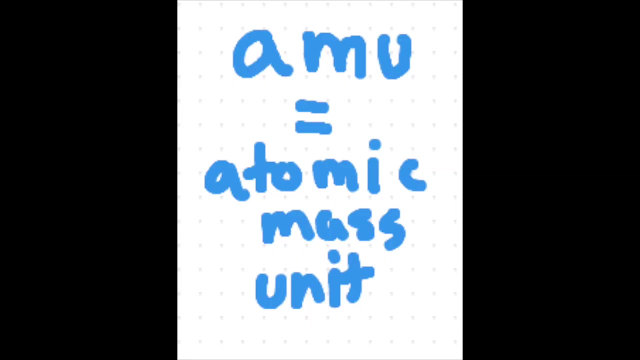 it. That's how big a mole is. but what exactly does a mole mean? In order to understand the mole, we have to go to our trusty periodic table, but before we do any calculations, we have to understand this one unit, the AMU or atomic mass unit. The atomic mass unit. 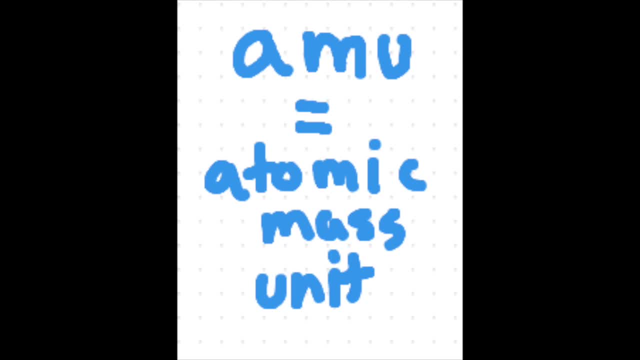 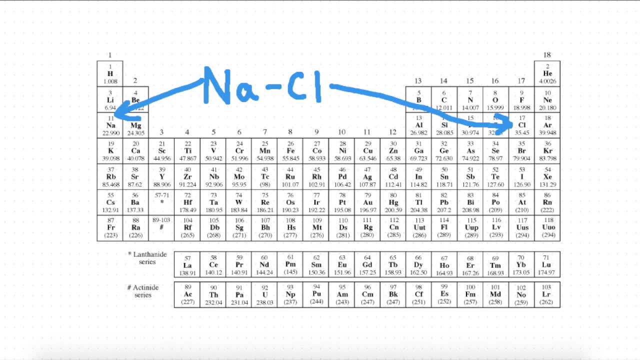 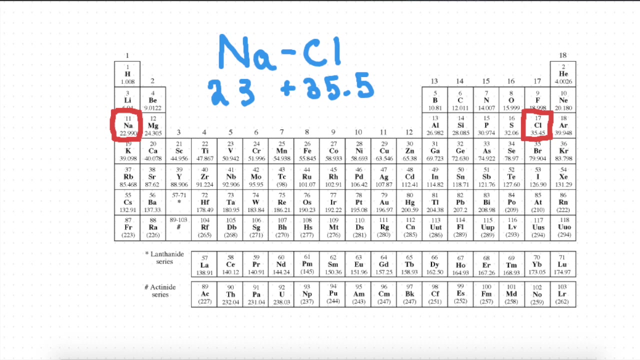 is just a way of measuring the mass of super small molecules. Anyway, let's say we have a salt molecule which is composed of sodium and chlorine. Sodium has an atomic mass of 23 AMU and chlorine has an atomic mass of 35.5 AMU, If you add. 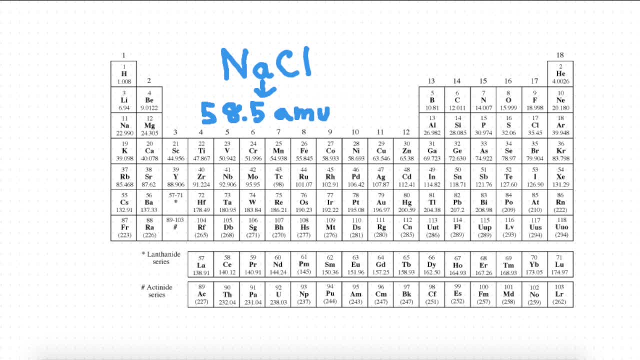 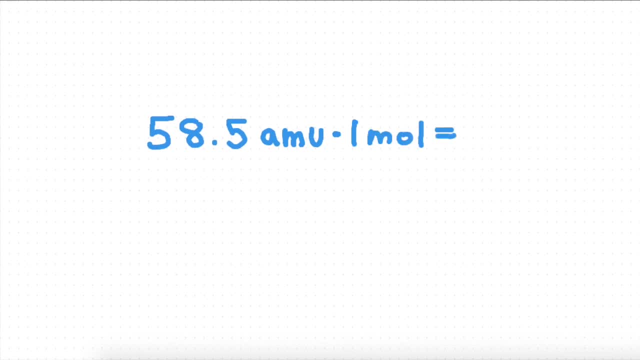 those up, you get 58.5 AMU. Now here's where the mole comes into play. If we take 58.5 AMU and multiply that to one mole, we get 58.5 grams. This is so big because now we turn units of AMU which we can't even see into grams. 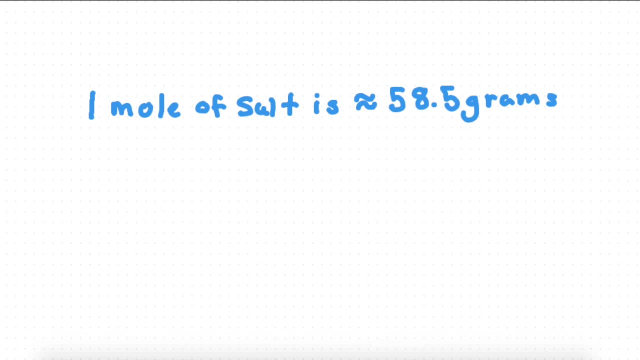 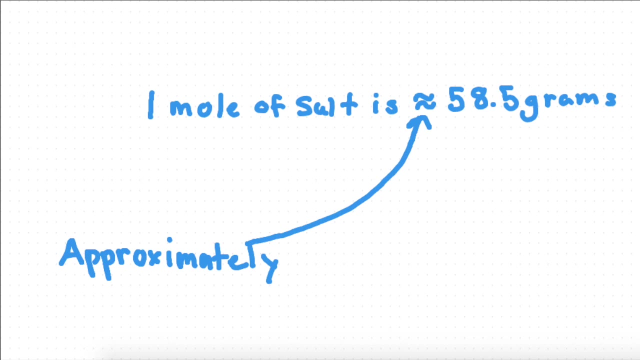 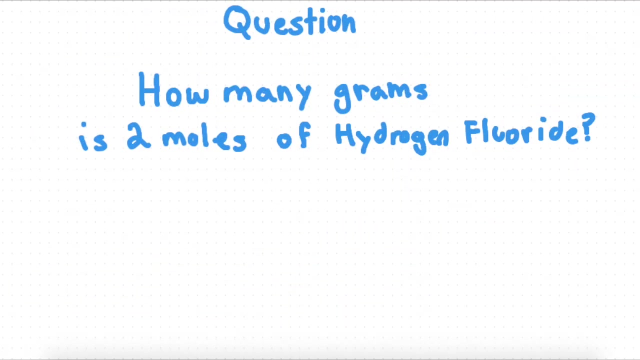 which we can even feel. So one mole of salt is 58.5 grams. By the way, that squiggly equal sign just means approximately, which means it's not exactly 58.5 grams, but almost that. Now I have a question for you: How many grams is two moles of hydrogen? 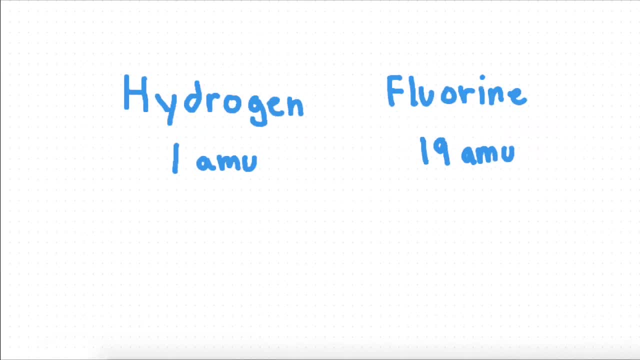 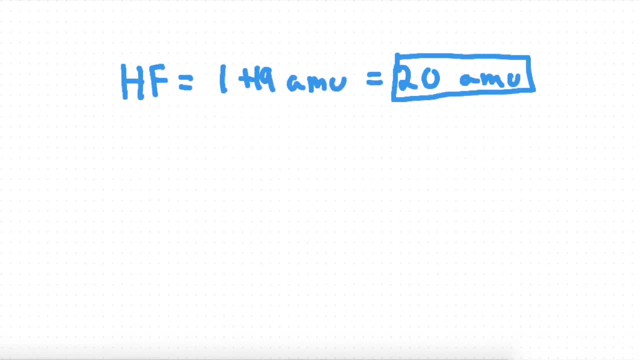 Hydrogen fluoride. Hydrogen is 1 AMU and fluorine is 19 AMU. Try to pause the video and figure it out yourself. Now let's all try to figure it out. HF, which is hydrogen fluoride, must equal 1 plus 19 AMU, which is just 20 AMU Now, since there's two moles. 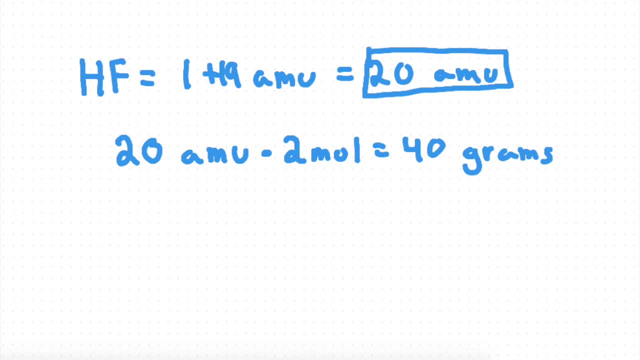